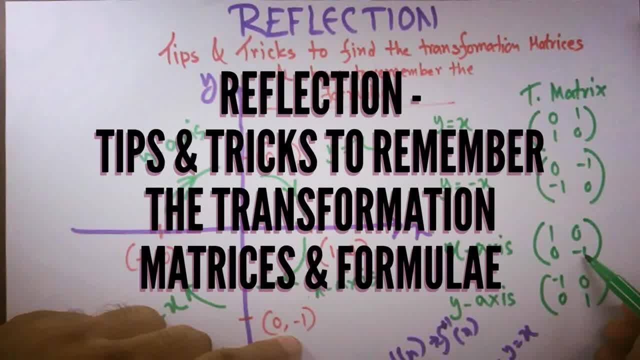 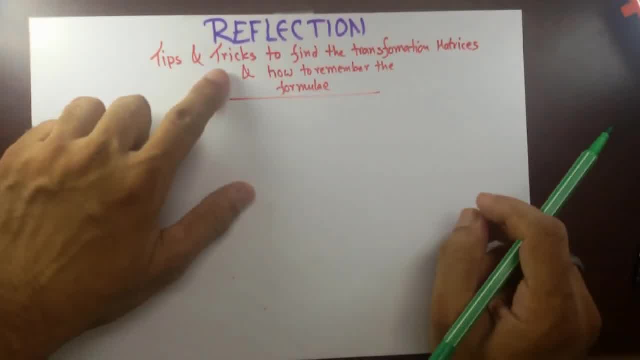 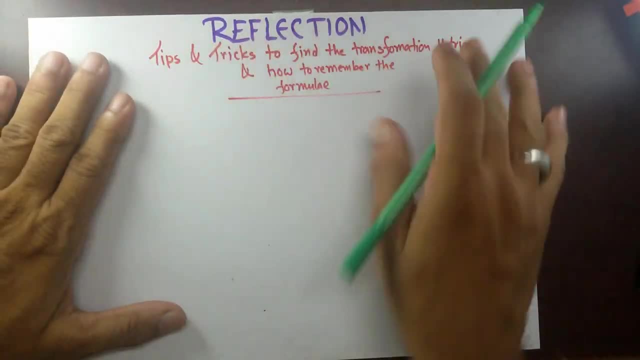 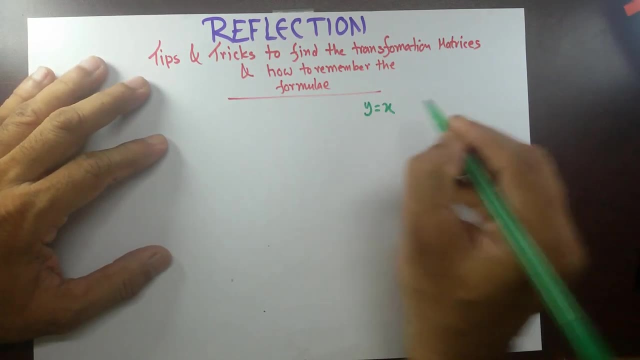 Good morning students. On today's lecture I'll give you some tips and tricks: how to find out the transformation matrices and how to remember the formula of reflection. Probably you remember that whenever we are reflecting one object on y equal to x, the transformation matrix would be 0, 1, 1, 0.. 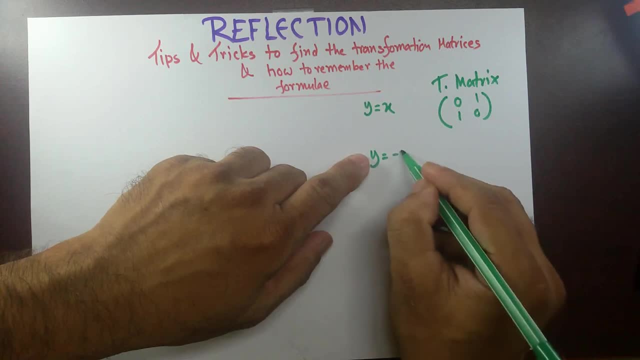 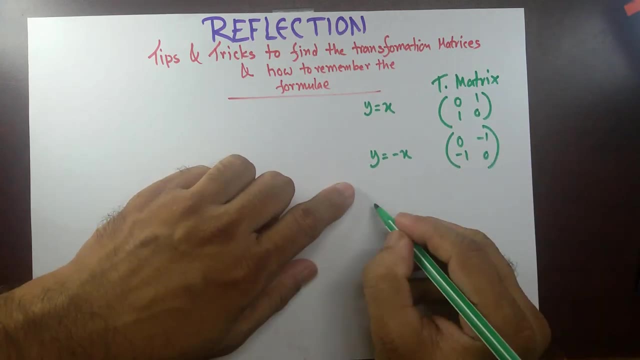 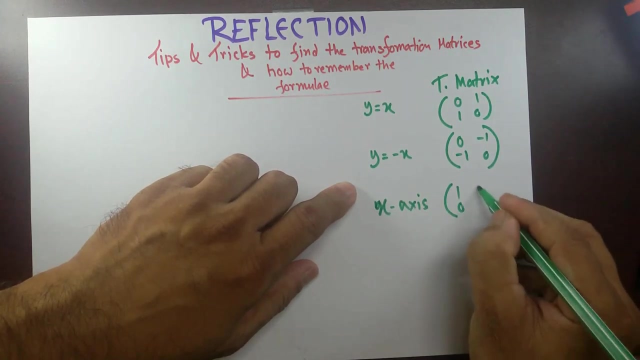 And when it's reflecting on y equal to minus x, then it's going to be 0, minus 1, minus 1, 0.. And when it's on x-axis, reflecting on x-axis, then it's going to be 1, 0, 0, minus 1.. 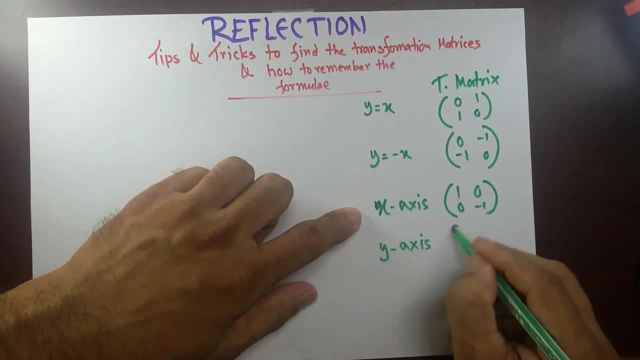 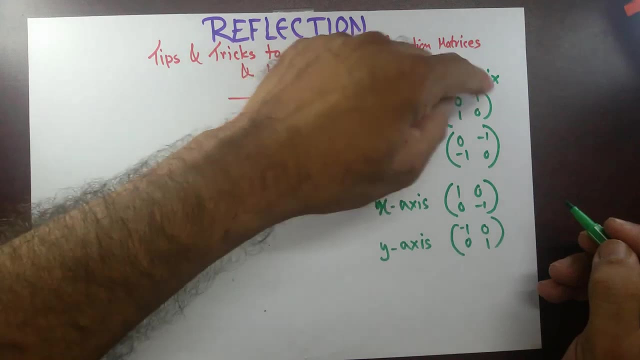 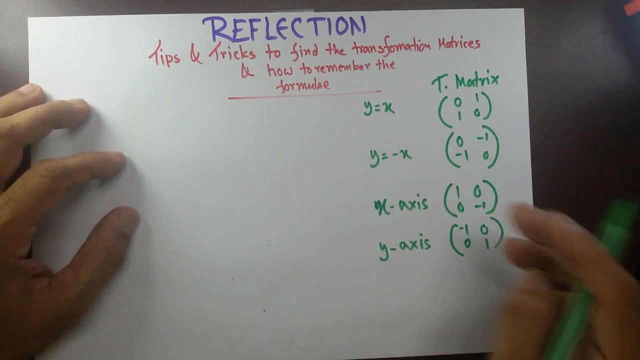 And when it's reflecting on y-axis, then it's going to be minus 1, 0, 0, 1.. Now there are only zeros and 1.. The problem is where to put zeros, where to put 1,, where to put positive sign, where to put negative sign. 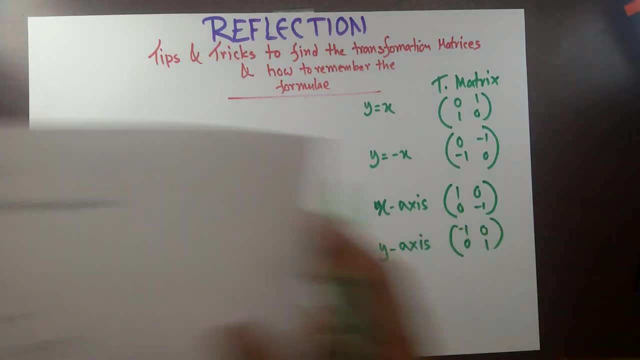 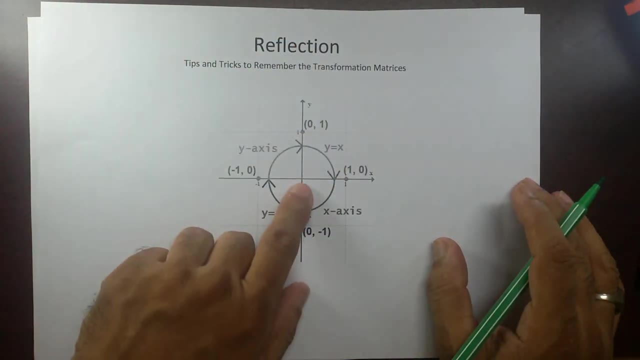 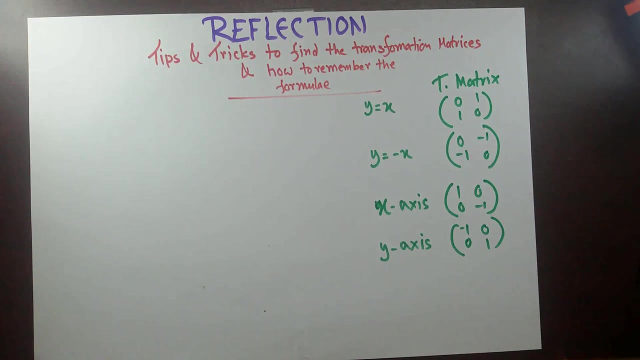 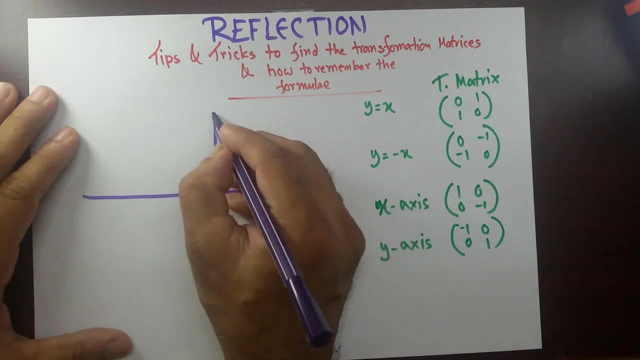 That's the problem. Okay, I have this printed out for you. Okay, See this grids x-axis and y-axis intersect at this point, And then these are the unit points. Okay, And I'm going to do that over here and show you how to just help you to remember that. 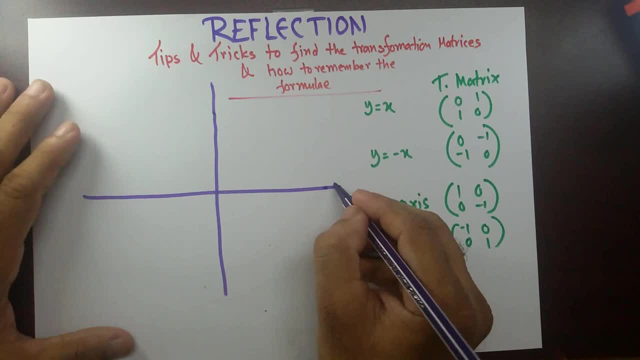 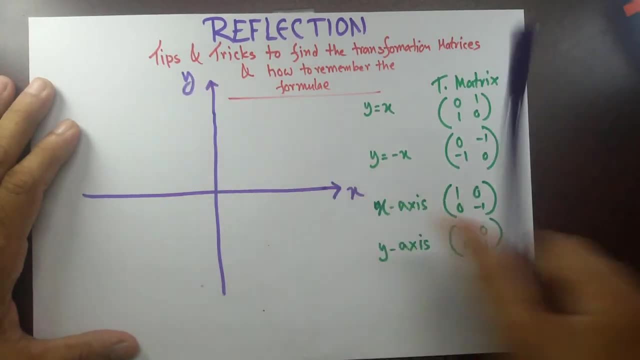 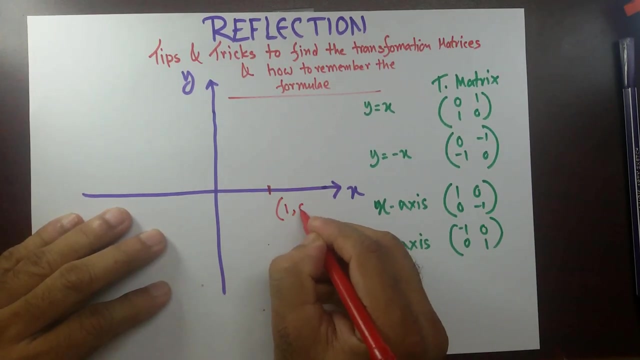 You don't need to memorize it, You need only to remember a few things to get this thing done correctly. Okay, This is one more question. This is x-axis, This is y-axis. Okay, So this unit point. it would be the coordinates of this point going to be 1, 0.. 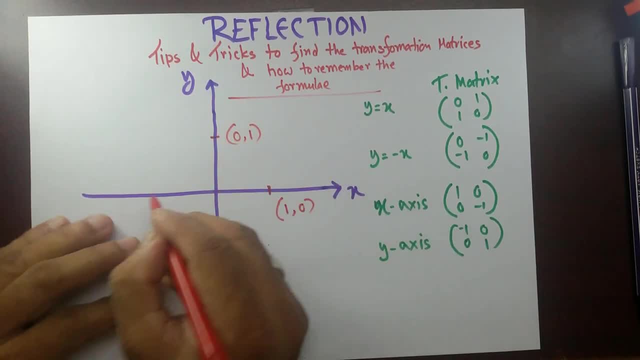 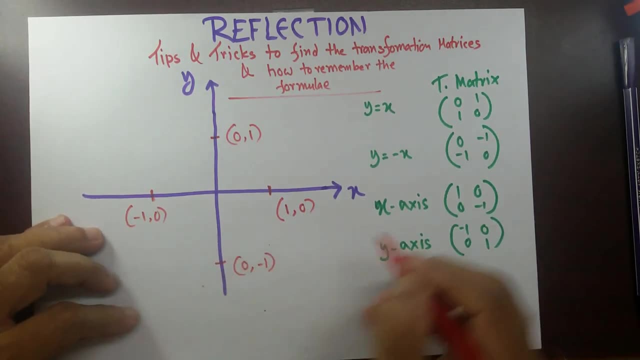 And over here it's going to be 0, 1.. This one over here is going to be minus 1, 0.. And this one is going to be 0, minus 1.. That's all you need to remember. 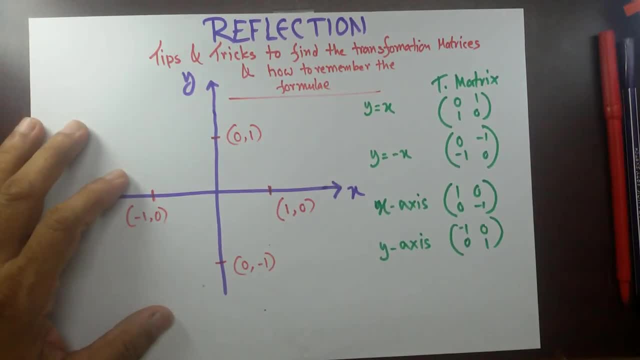 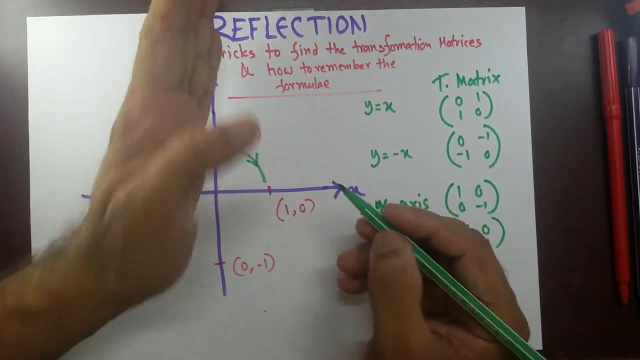 Okay, And then for reflection, what are you going to do? We're going to go. We're going to go. clockwise rotation: Okay, We are going from this way to that way: North to east, Eastward and eastward to the southward. 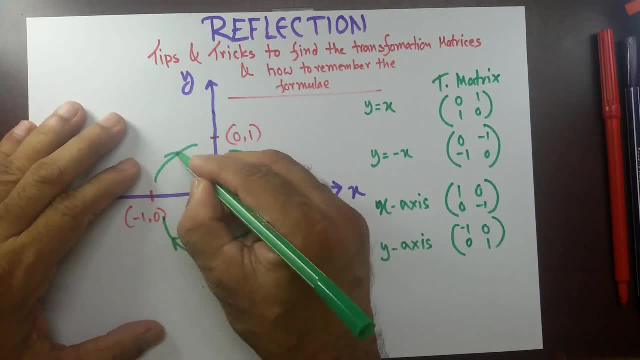 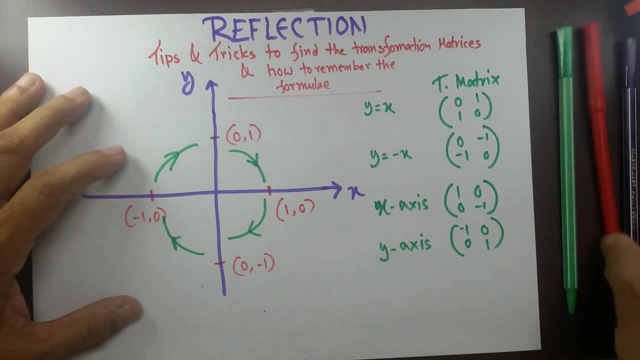 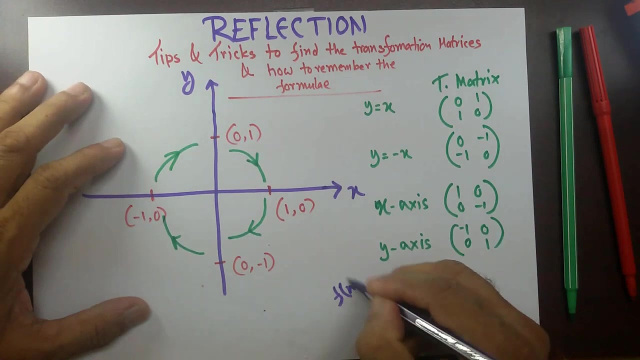 Southward to westward And westward to northwards. Okay, This is how we're going to do that. Okay, Now I hope in the functions you have seen that every function- okay, graph of function and its inverse, okay, its inverse- they reflect on function and its inverse. 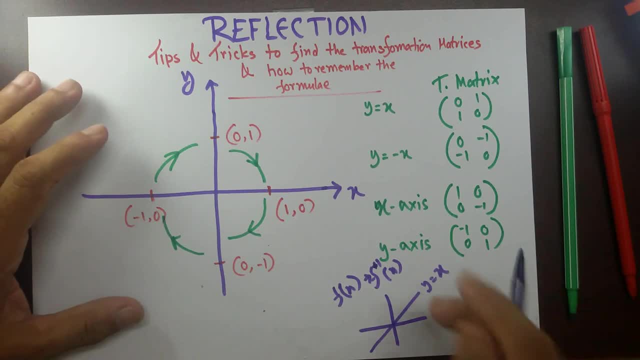 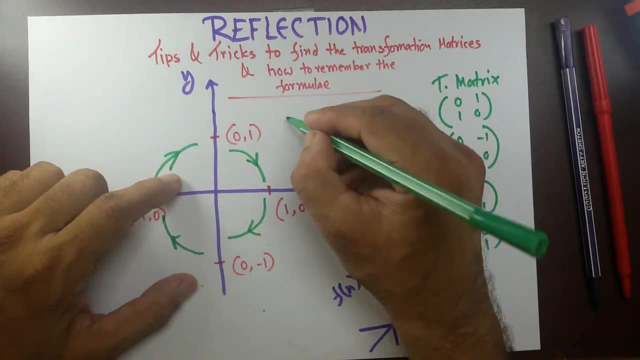 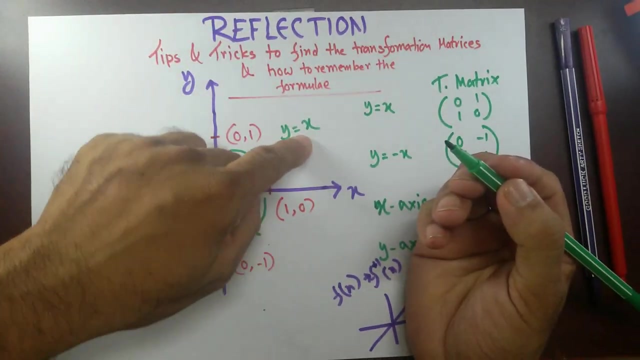 it's reflect on y equal to x-axis. Okay, I like to remember this thing. Okay, Now think this is: y equal to x-axis, y equal to x-axis, right over here. Okay, In the first quadrant, This is you need to remember. 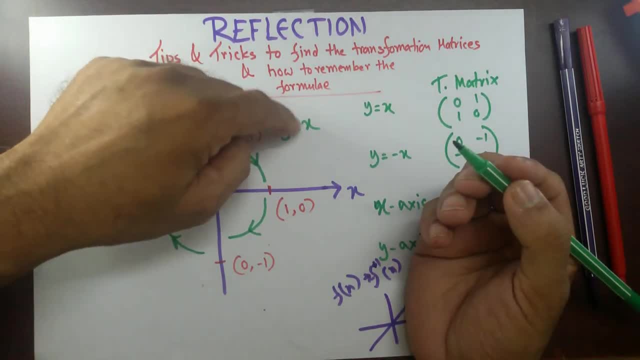 And opposite of this. This is y equal to x-axis. This is general knowledge, Okay, Only thing you need to remember. first quadrant, write down y equal to x. On the opposite, just write down y equal to minus x. Okay. 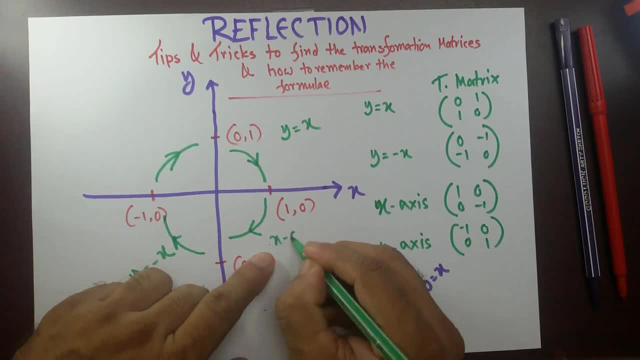 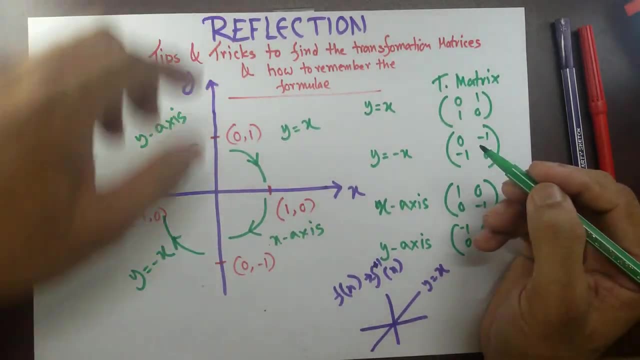 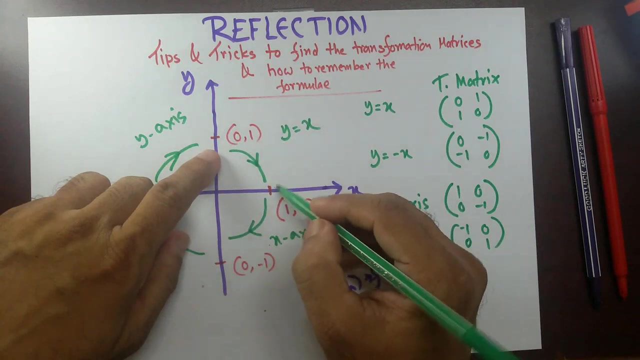 And this fourth quadrant, write down x-axis And, opposite of this, of course, y-axis. Now, if you are reflecting your object on y equal to x-axis, Now the transformation matrix going from this place to this place, Unit is 0, 1 to 1, 0.. 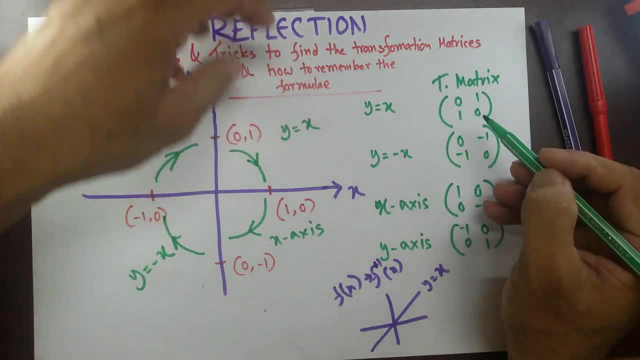 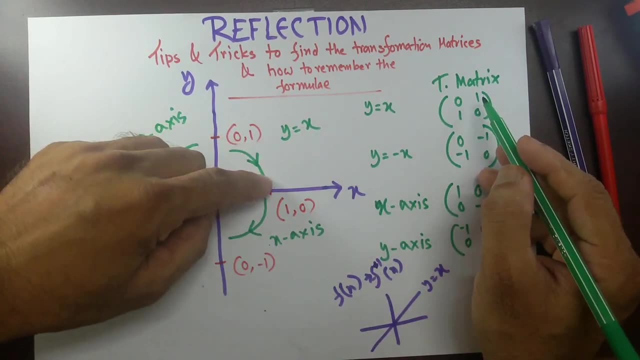 Look at this: 0, 1 to 1, 0.. Okay, So whenever any object is reflected on y-axis, y equal to x-axis, then you use this transformation matrix and you remember this way. Same way, if it's y equal to minus x-axis where it's reflected, then from here to here: 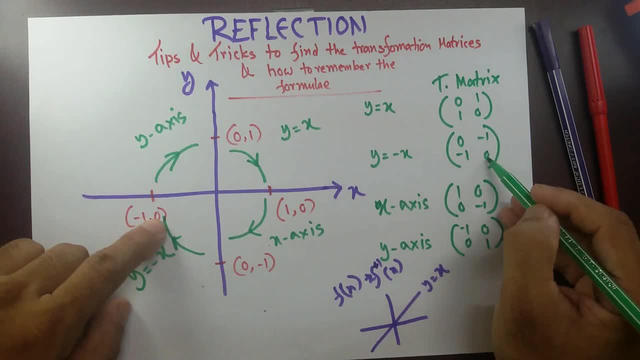 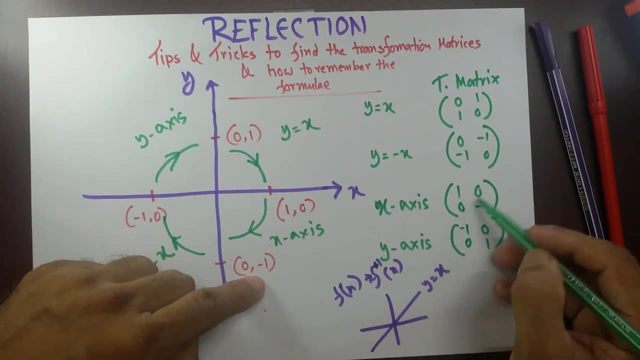 0 minus 1, 0 minus 1, minus 1, 0, minus 1, 0.. If it's on x-axis from here to here, 1, 0 to 0 minus 1, 1, 0, 0 minus 1.. 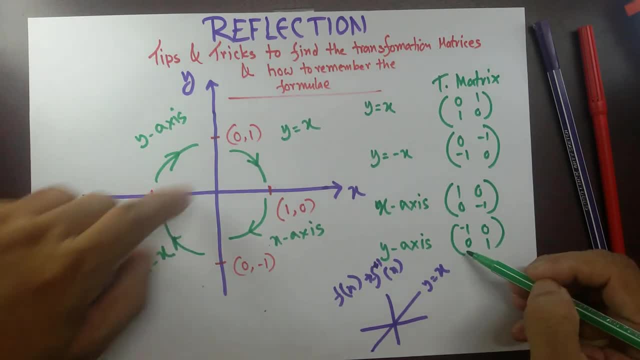 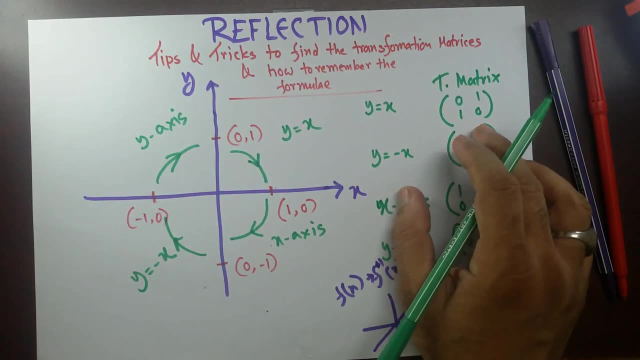 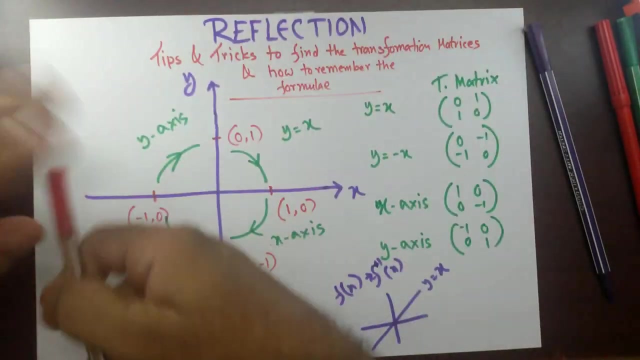 And for y-axis minus 1, 0 to 0, 1.. Okay, This is how you remember the transformation matrix. And whenever it comes to formula, okay, take a point. Take a point. Let's say I have this point over here. a, b. 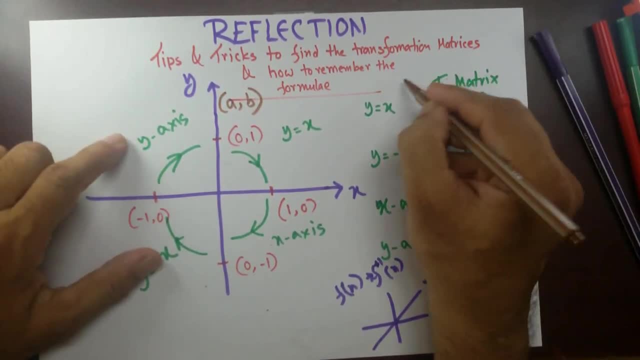 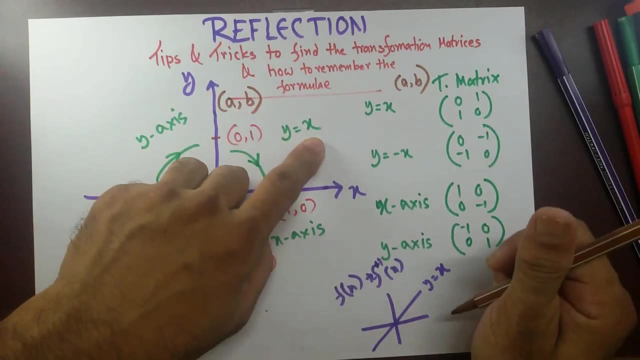 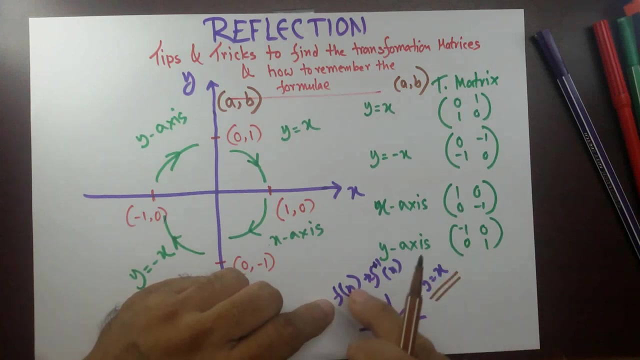 Okay, Point a- b, And if the point is a- b, And if you are reflecting on y equal to x-axis, Okay, If you are reflecting on y equal to x-axis. Remember this thing Whenever you have this function, an inverse function, reflected on y equal to x. 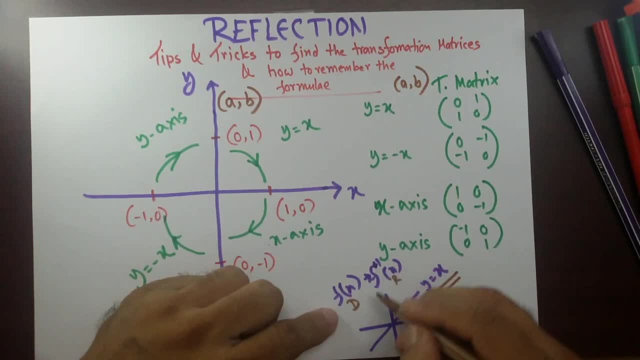 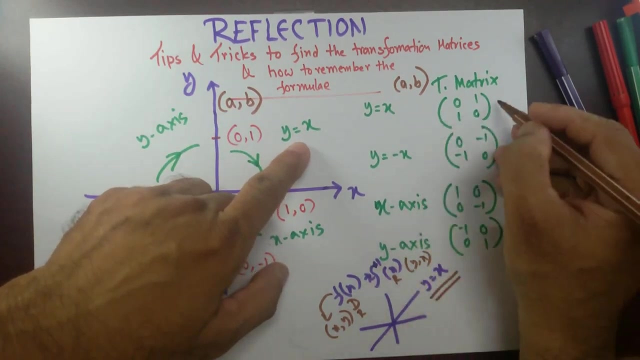 the domain of the function becomes the range of the inverse, and range of the function becomes the domain of this inverse. Okay, So what actually means x and y coordinates of this function? it becomes. It becomes y and x. Okay, So whenever we are reflecting on this one, the formula is going to be b- a. 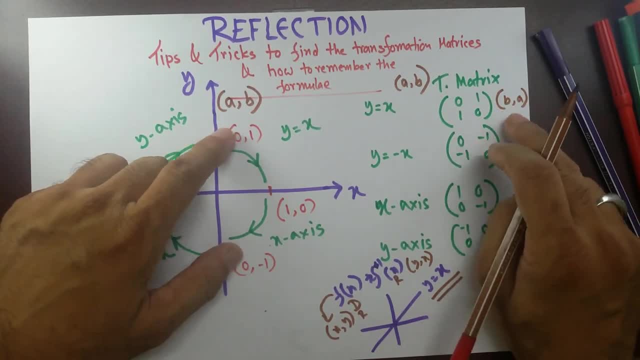 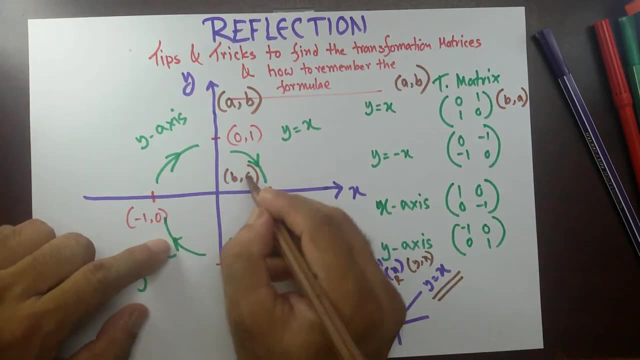 All right, X coordinates is going to be changing. It's going to be b a, So I can write down this one b a over here And whenever it's opposite, okay, same way. just what you need to do. 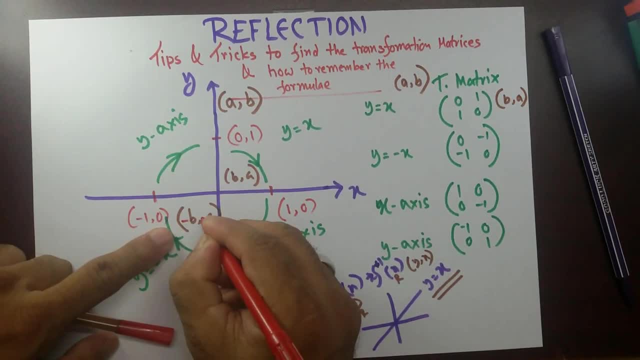 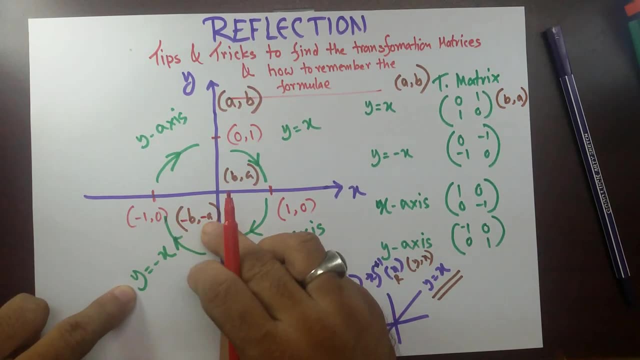 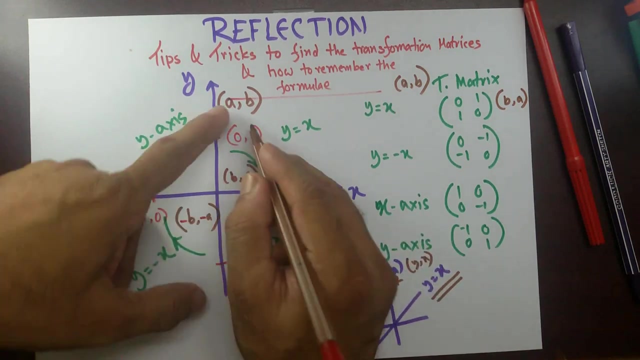 you just need to put negative sign before that. Okay, So this is b a, And whenever you are reflecting on y equal to minus x, it's minus b minus a Over here. okay, this a b over here. see, I'm going to have this a. 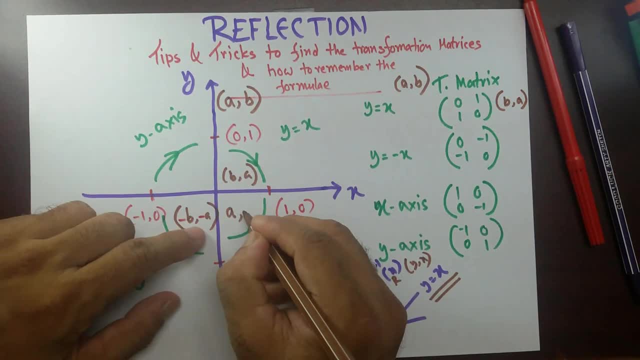 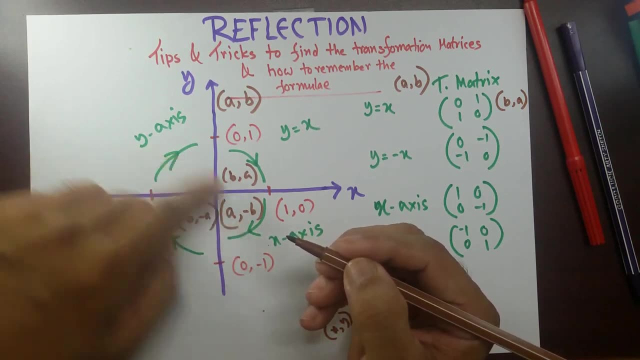 Okay, a, But below x-axis y coordinates is negative. So this is a minus b. Okay, And whenever you are going to the opposite, vertically opposite on y-axis, then over here, same way: a and b. But. 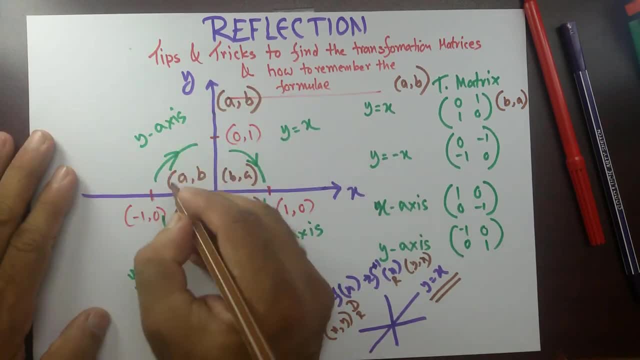 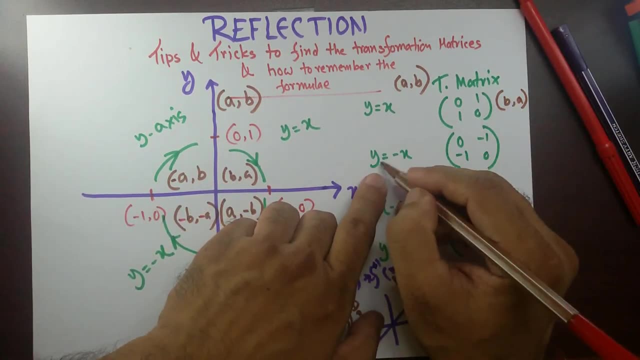 Since it's the x-axis on the left-hand side of the y-axis, it's negative. So it's negative minus a, b. So y minus x. whenever reflected y equal to minus x, then this is going to be minus b minus a. 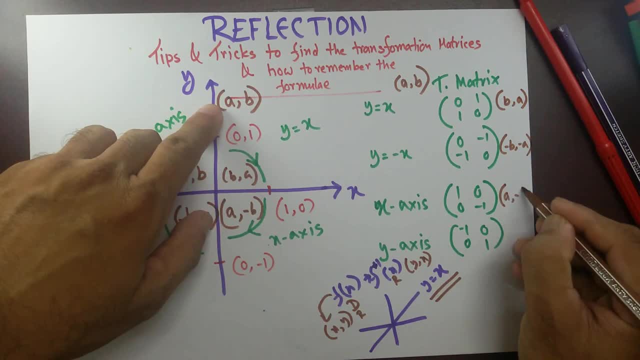 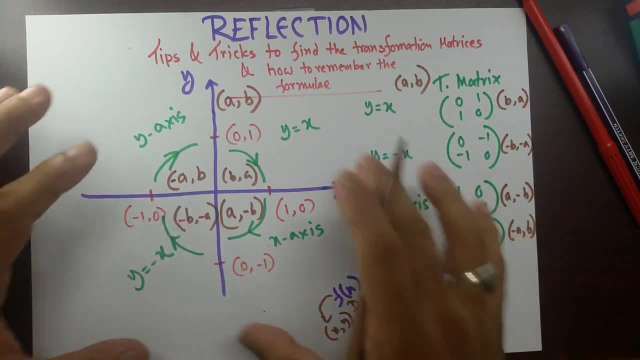 And on x-axis it's going to be a minus b, And on the y-axis it's going to be minus a- b. If you just give a little time and look it over, all right, then it's going to be very easy for you. 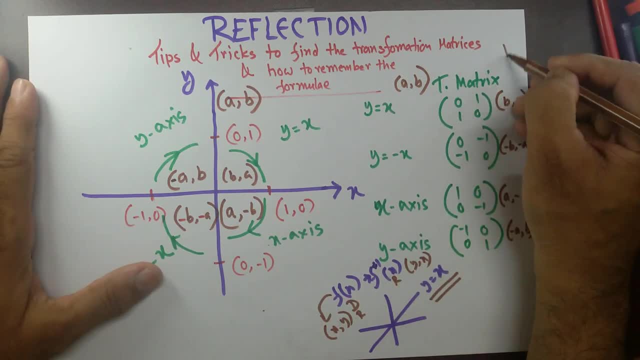 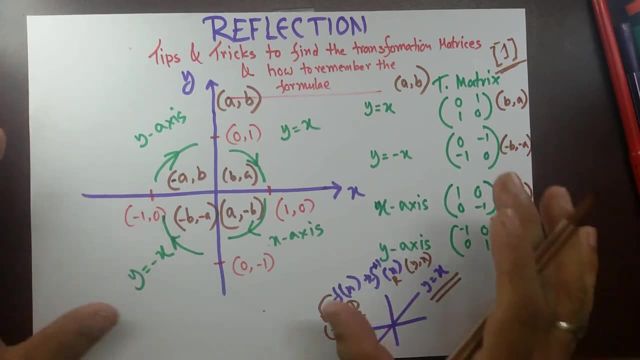 It's one-mark's question. Each of them one-mark's question. Okay, But one-mark is one-mark. Okay, That's going to be make the difference a star to a Okay. So hopefully this is going to be helpful to you.